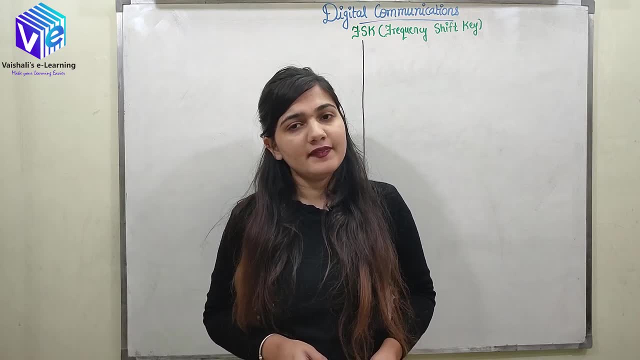 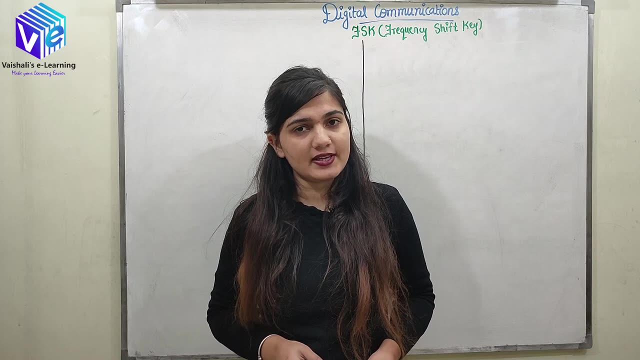 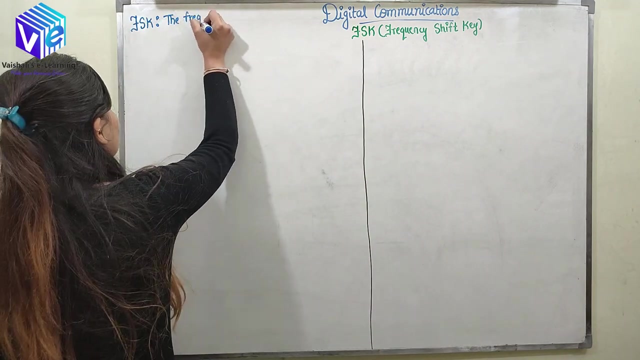 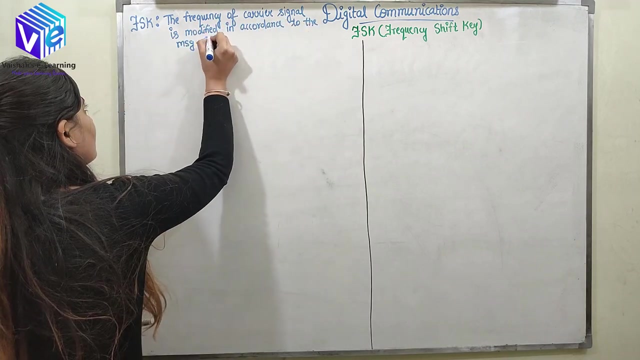 Then we will discuss the transmitter block diagram, Then we will come to the receiver block diagram and at last we will see the constellation diagram of FSK. So let's begin our discussion with the definition of FSK. So, according to the definition, the frequency. 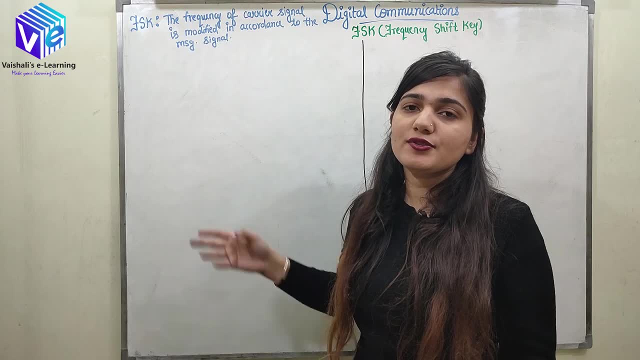 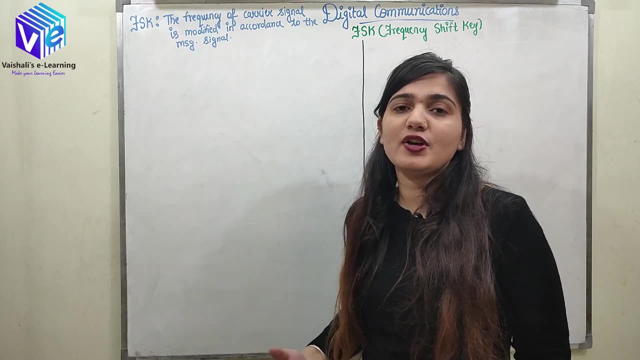 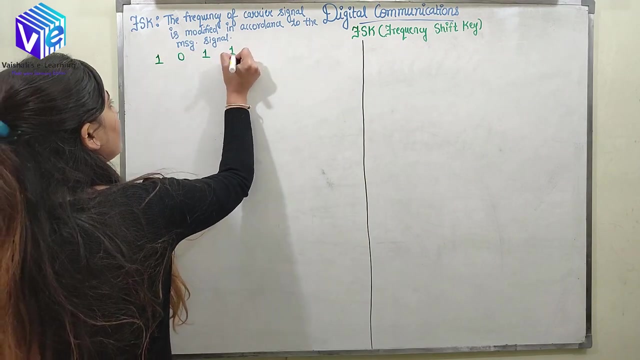 of the carrier signal is changed in accordance to the message signal. So when the message signal is changed, at that time the frequency of the carrier is also changed. So let's see this thing with the help of an example. So I will take an example. So this is my. 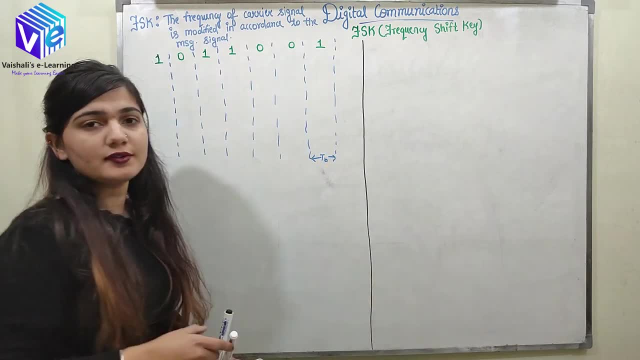 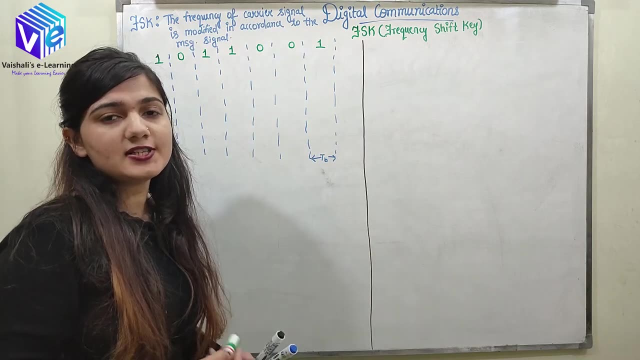 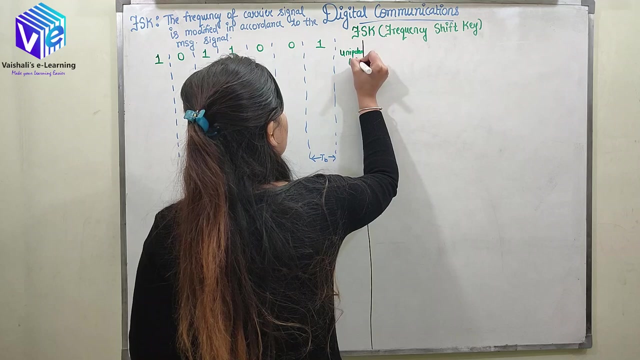 bit duration, which is TB. So now, this is my message signal, which is digital message signal 011001.. So now, if I represent this digital signal with the help of line encoding and I make the unipolar NRZ line encoding technique, So, according to unipolar NRZ 1, 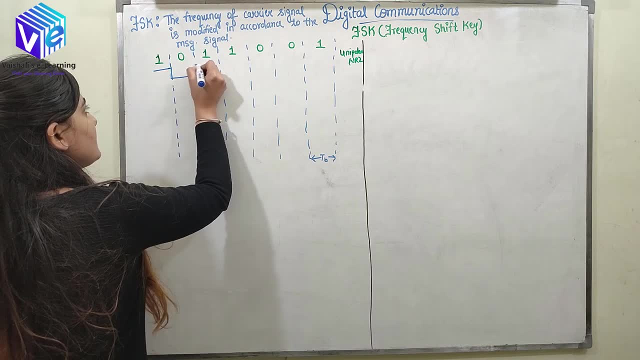 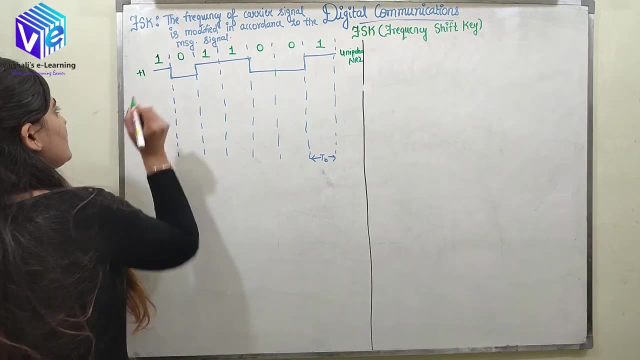 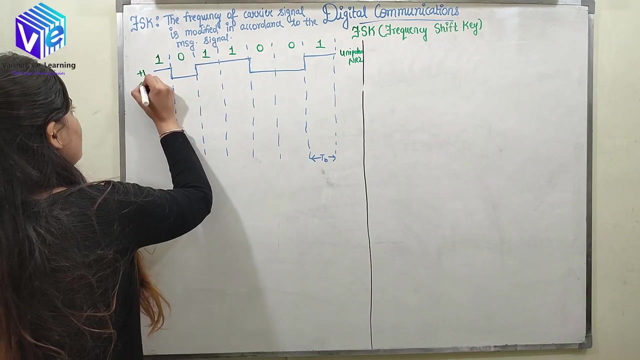 is represented by 1 and 0 is represented by 0. So here I am taking a generalized case where I am taking the positive voltage to be plus 1. So when I have this signal, I can represent it with the help of plus 1 and 0. So now I have a carrier signal. So in 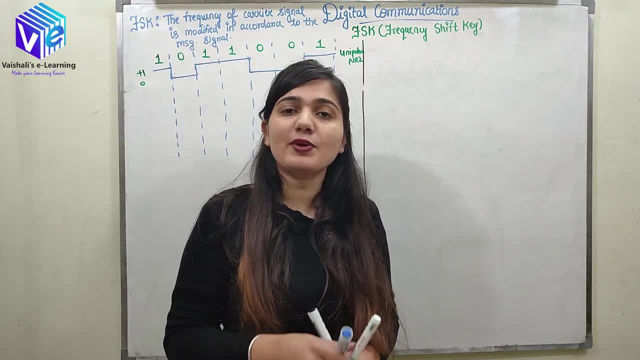 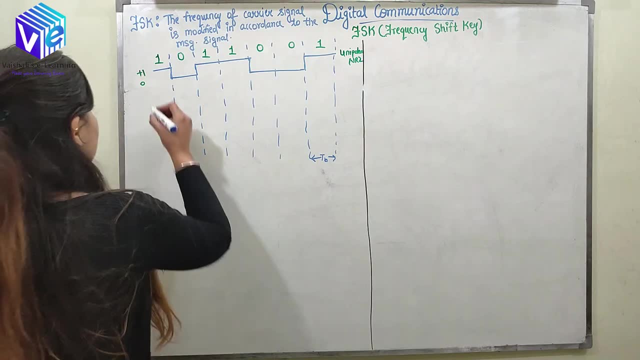 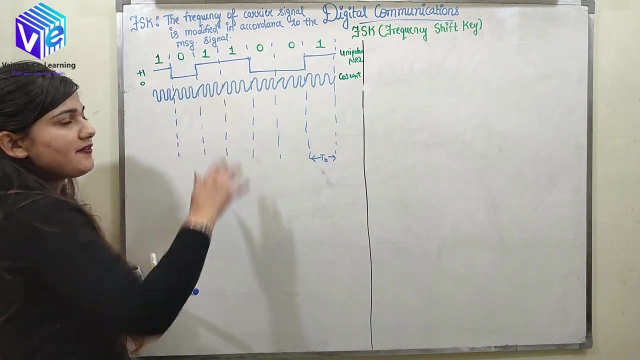 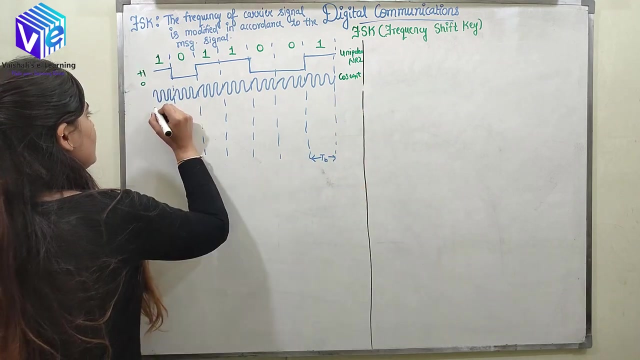 frequency modulation scheme. I will take two carriers. So first carrier is having high frequency and the second carrier is having low frequency. So this is my high frequency carrier and I represented it with cos omega L. Now coming to the low frequency carrier, 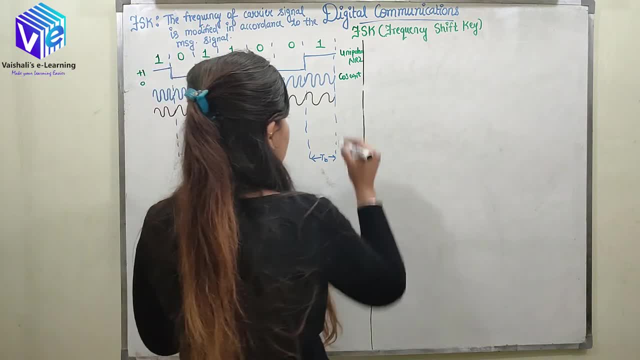 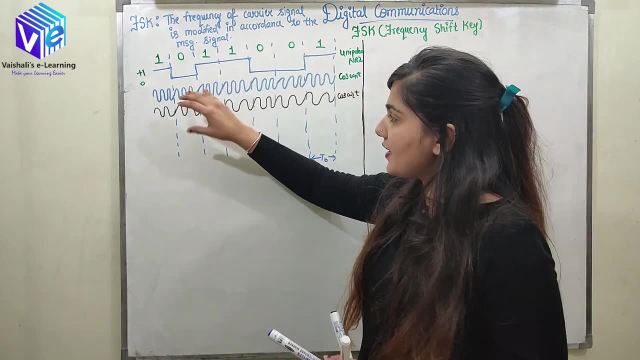 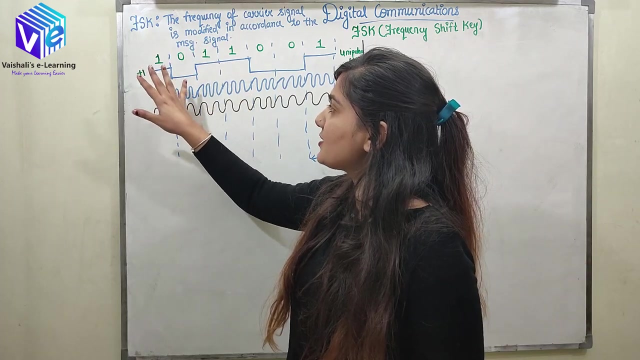 So this is my low frequency carrier, So I will represent it with cos omega LT. So now coming to the frequency modulation. So when I modulate these carriers according to my data, So at that time I can have a projection scheme where one is represented by high frequency. 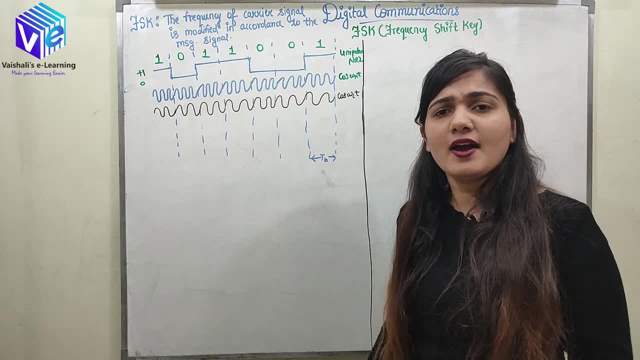 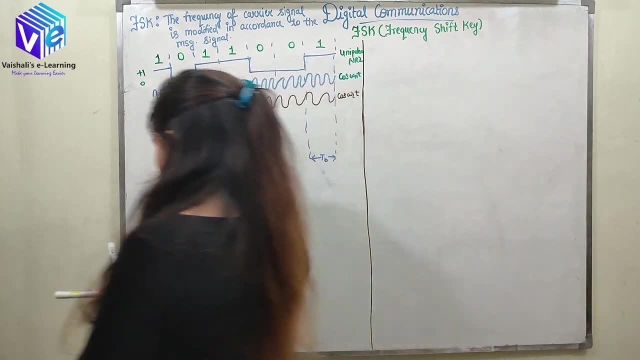 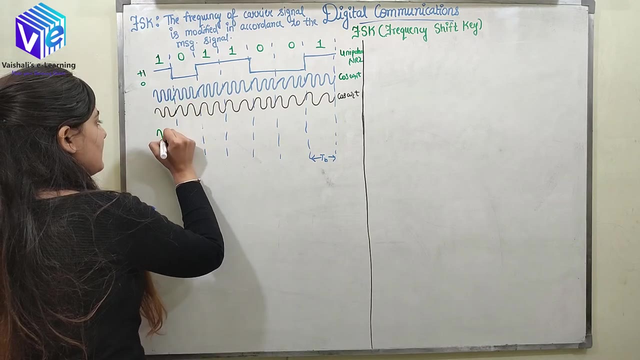 carrier and zero is represented by low frequency carrier. How we will achieve this we will discuss later, but let's suppose here one is represented by high frequency carrier and zero is represented by low frequency carrier. So wherever I have one, I will represent it with high frequency, and wherever I have zero, 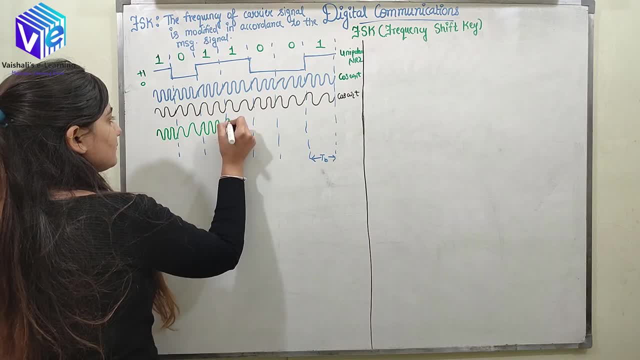 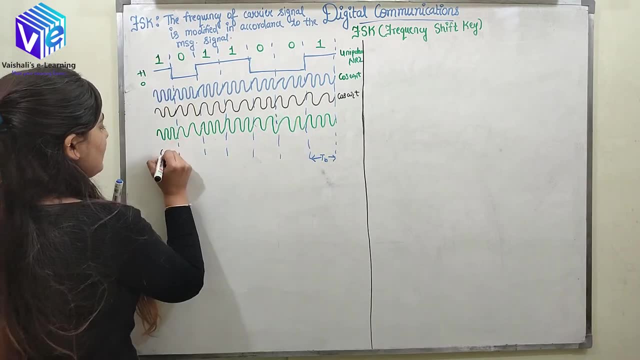 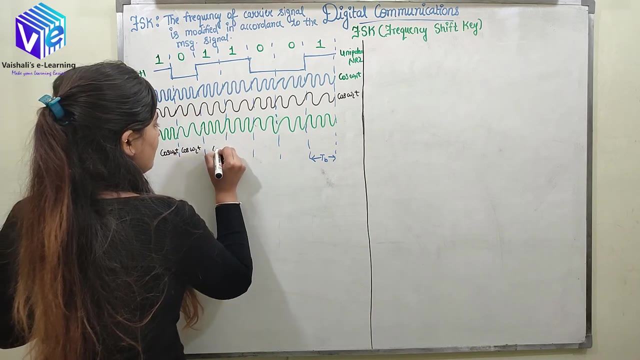 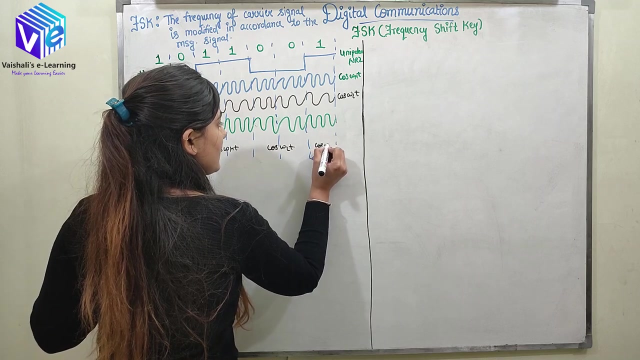 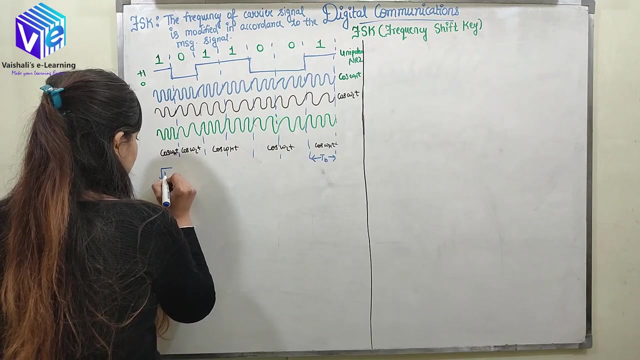 I will represent it with low frequency. So here I have one. it is represented by cos omega HT, zero by cos omega LT, one one cos omega HT, zero, zero by cos omega LT, one by cos omega HT. So now I have this message signal which has, which is represented by under root PS into 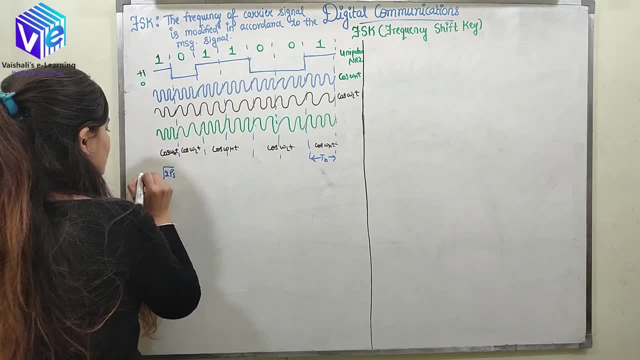 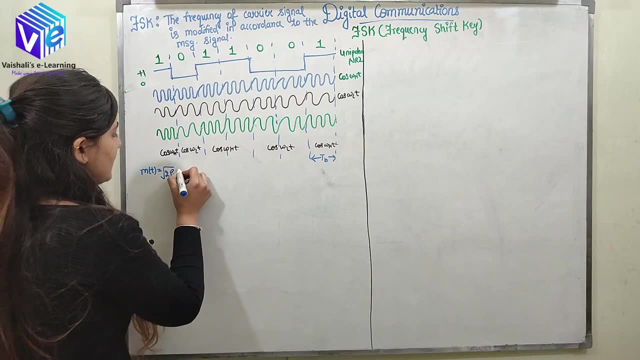 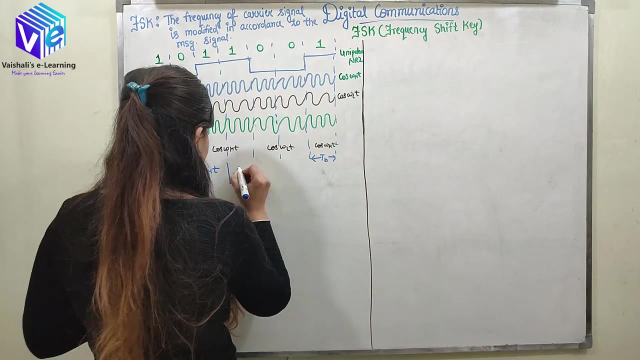 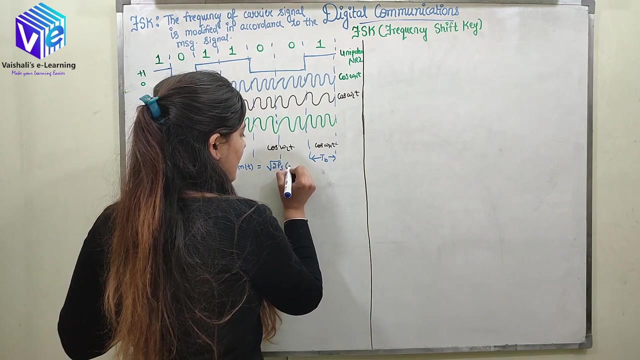 two Under root 2 PS. So this message signal is represented by under root 2 PS. So it is multiplied by cos omega HT when it is one, and message signal is again under root 2 PS. So amplitude is represented like this and the carrier is now cos omega L. 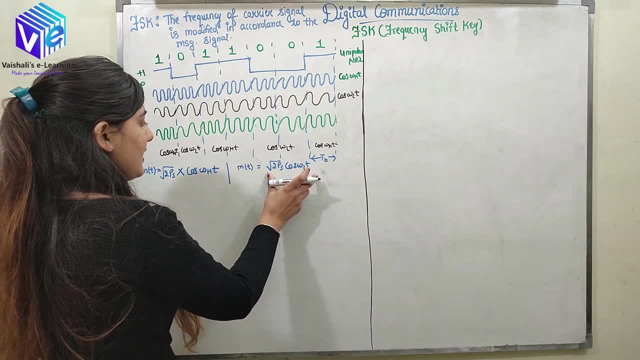 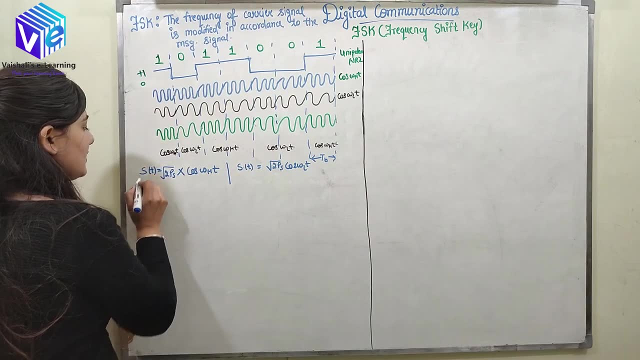 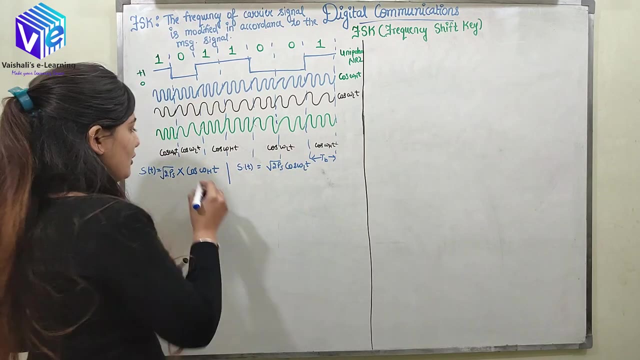 So at zero, the message signal is represented like this. So now this is my. when I multiply this, this is my output, ST, which is the modulated output. So when signal is multiplied by the carrier, again the signal is multiplied by the carrier. So this case is for 1 and this case is for zero. 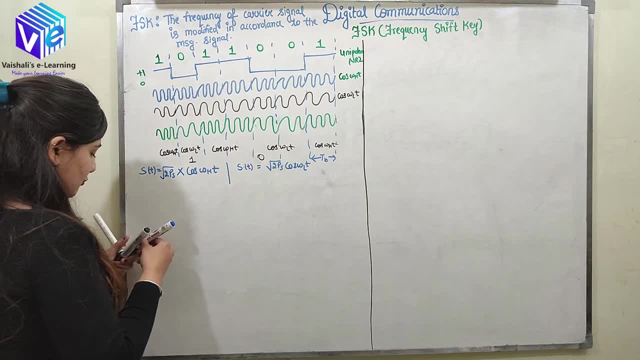 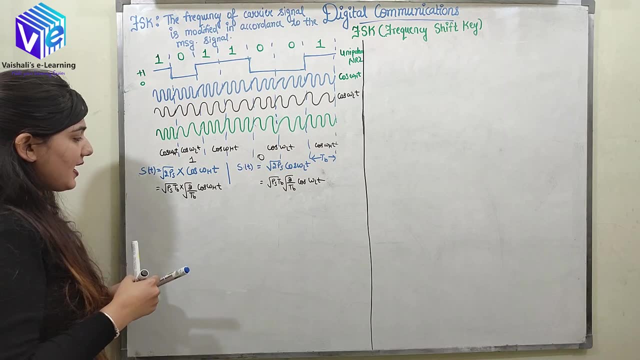 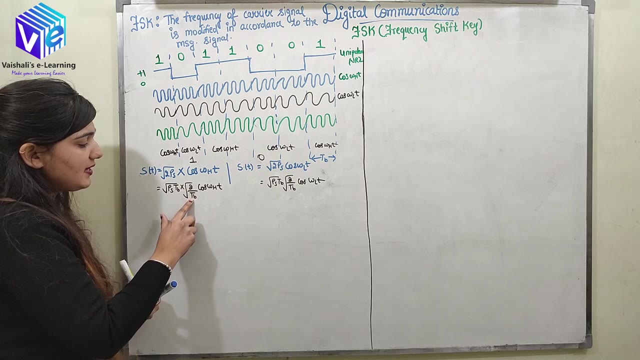 So now what is happening? I can write under root 2 PS as Let's see for what it is, Okay. Okay, write my under root 2 PS as PS into TB divided by TB, so TB and TB can cancel out, and I left out with under root 2 PS only, so this and this are equal. I hope now. 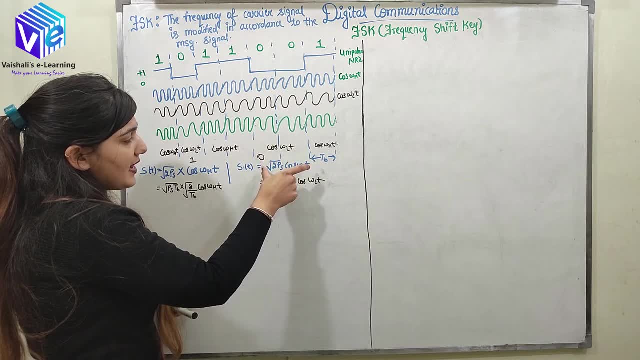 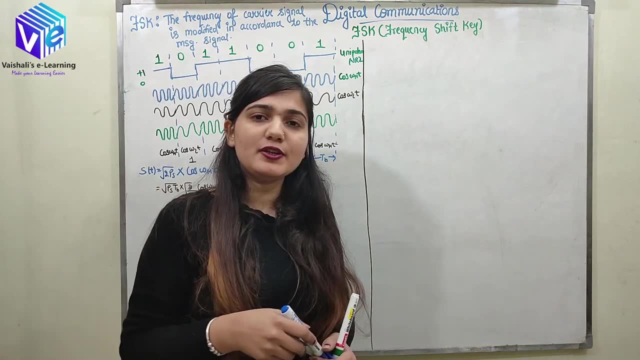 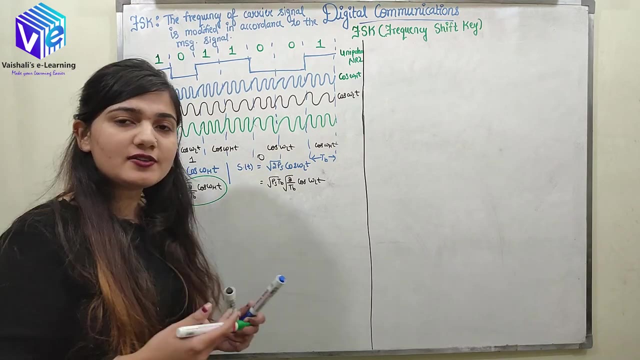 you can see. similarly, the lower carrier, lower frequency carrier, are represented like this. so now from my previous video, you can watch my previous video and you can see that this function is representing an orthogonal function. orthogonal is a function which is having a unit energy, so I represented there. I 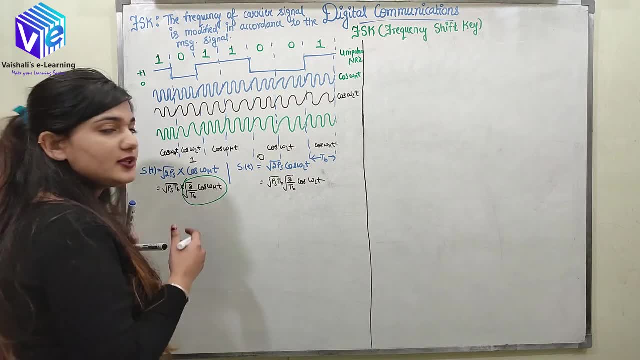 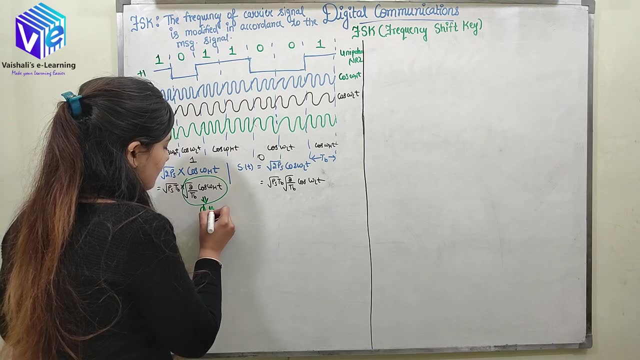 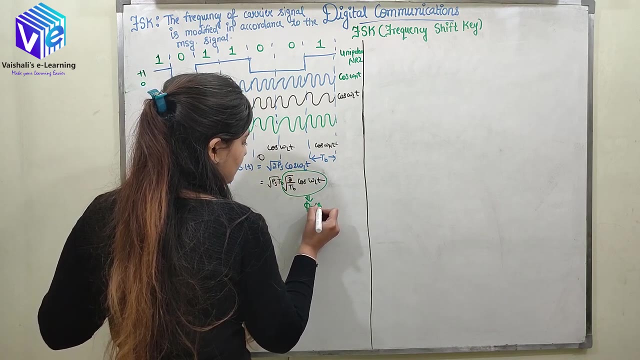 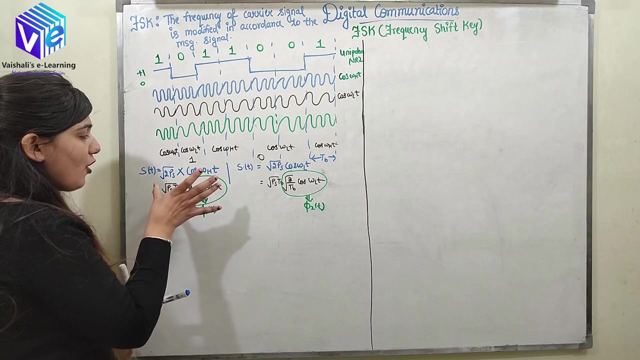 integrated it and I show you that how the signal is having unit energy. so now this is my orthogonal function first. so I am representing it with phi 1 T. this is my orthogonal function. 2, I am representing it with phi 2 T. so now my output. the output would be composed of this signal plus this: 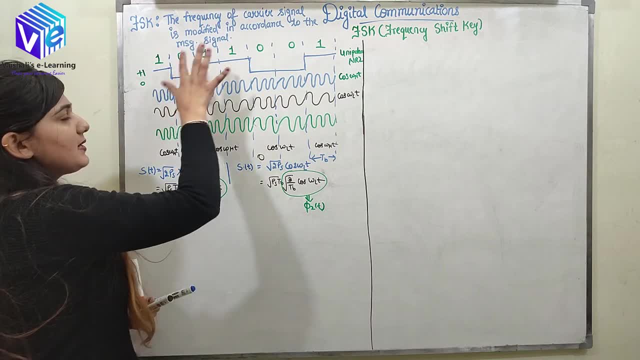 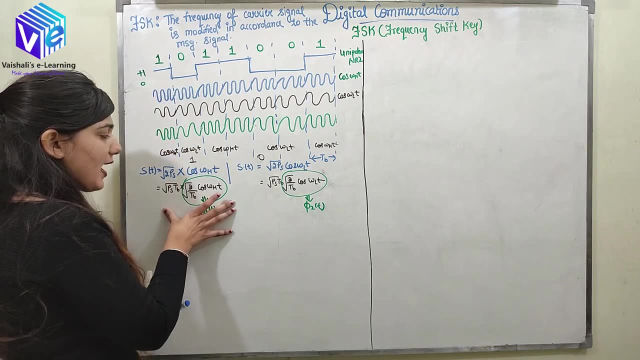 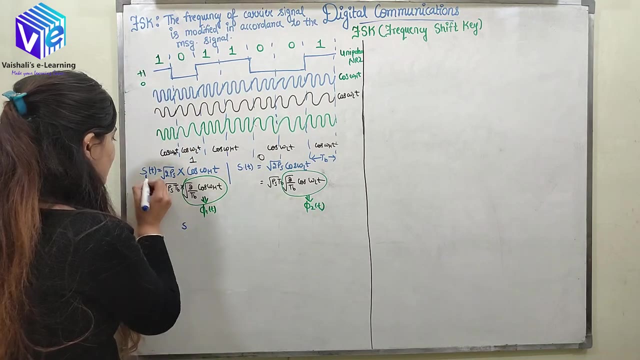 signal. so my output is composed of 1 plus 0, so some at some part it has 100, some part it has 0. so at the output I should have the representation for 1 as well as the representation for 0, so the output ST. so this was my s1 T and this. 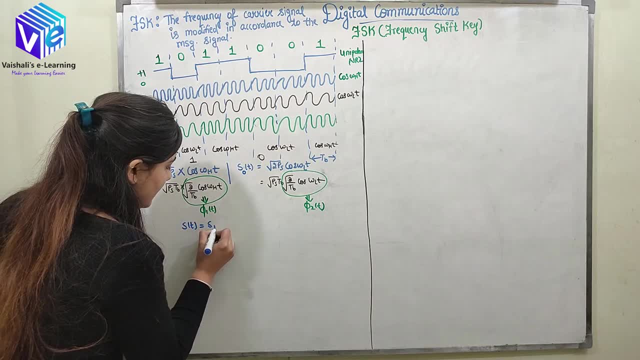 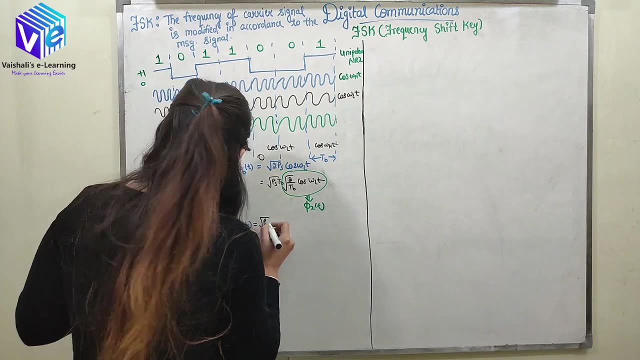 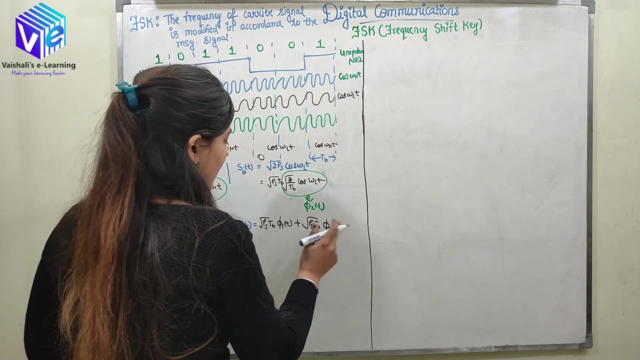 was my s0 T. the output ST is equal to s1 T plus S0T, So output is represented like under root PSTB phi1T plus under root PSTB phi2T. So I can represent it as EB. So in. 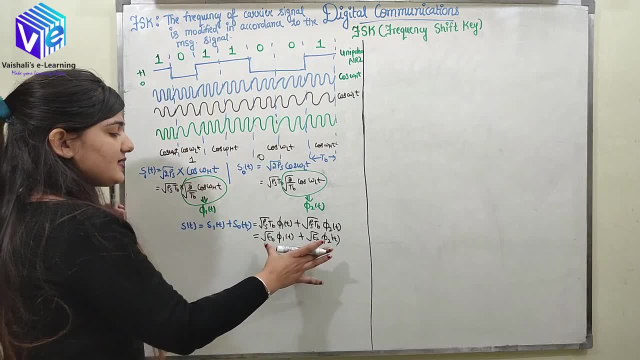 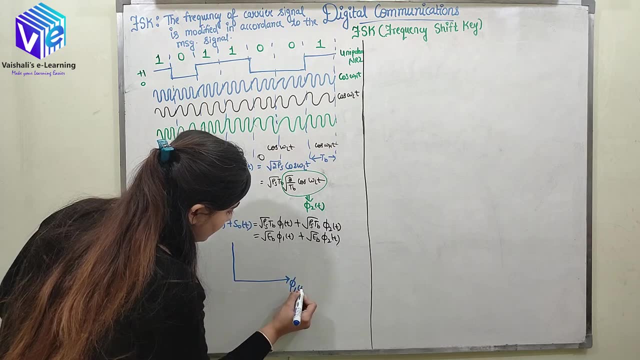 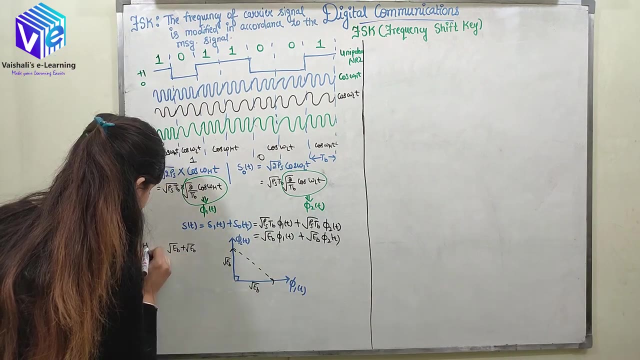 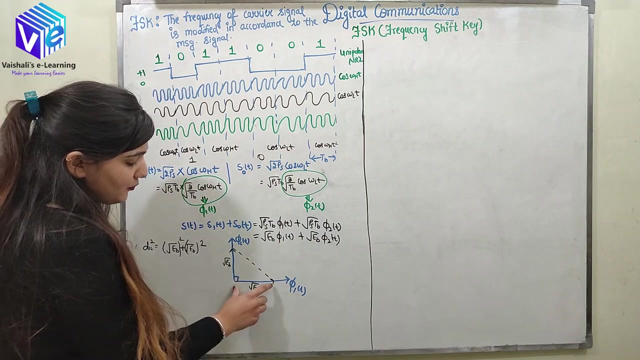 the terms of energies, my FSK signal is represented like this: So if I make the projection on phi directions, So according to the projections on phi direction, in phi1 direction the projection is under root EB and in phi2 direction also. 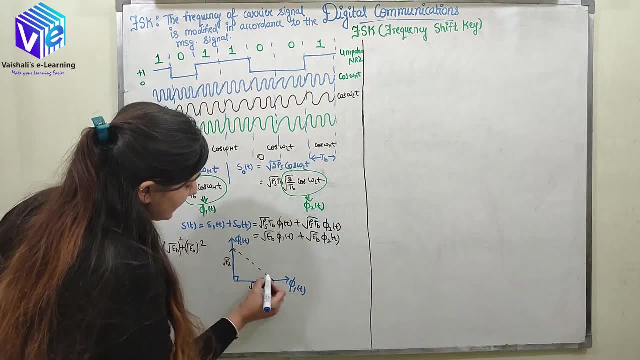 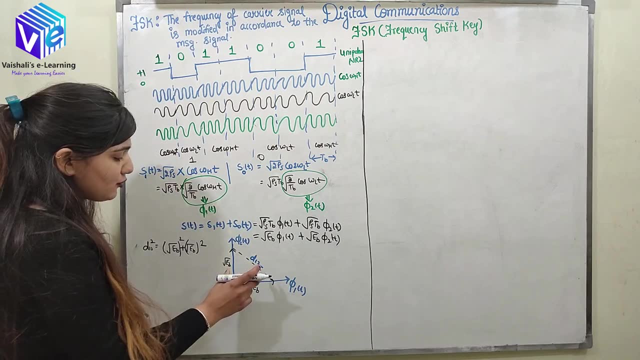 the projection is under root EB. So if I have to take the distance, D12.. So I will see this right angle triangle and in this right angle triangle I will see this right angle triangle. I will use the Pythagoras theorem. So, according to the Pythagoras, 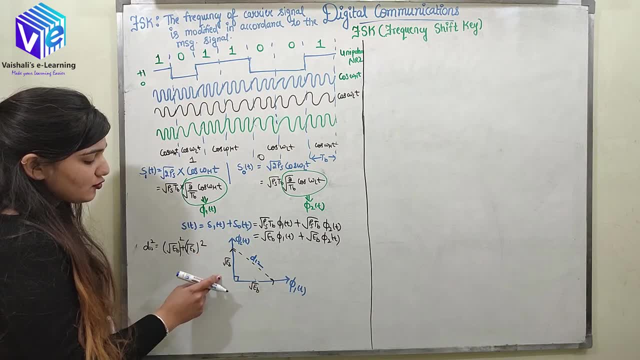 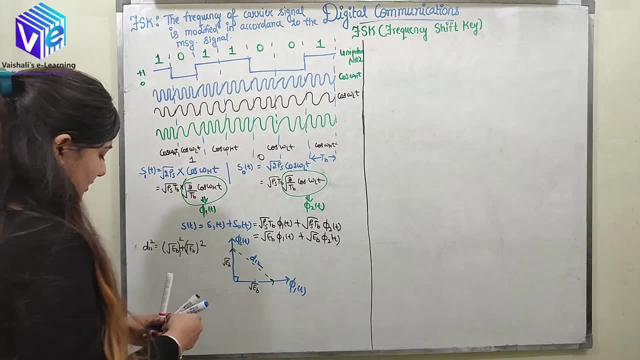 theorem. the hypotenuse square is the summation of the square of the sides. So D12 square is equal to under root EB square plus under root EB square. So so D12 is equal to under root 2EB. So. 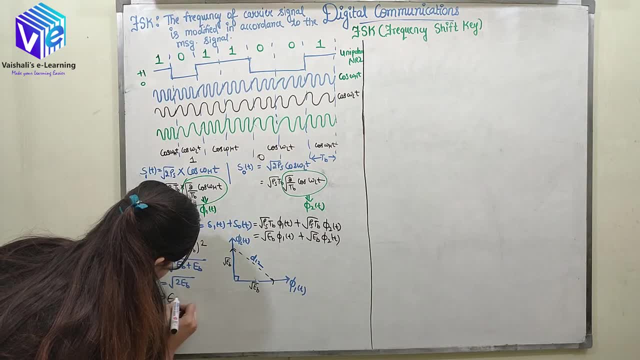 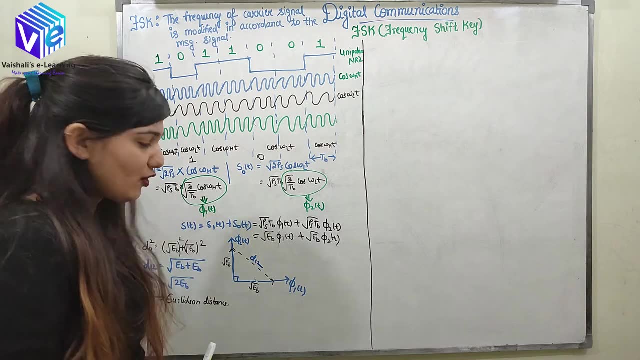 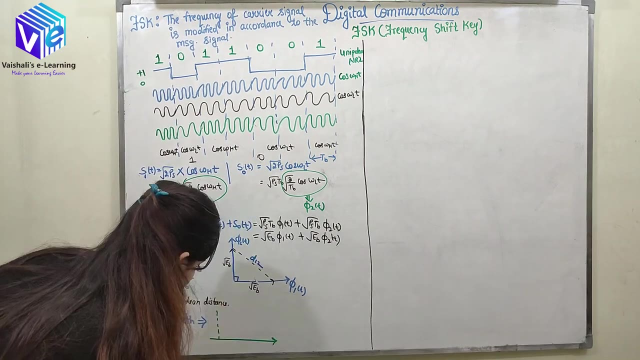 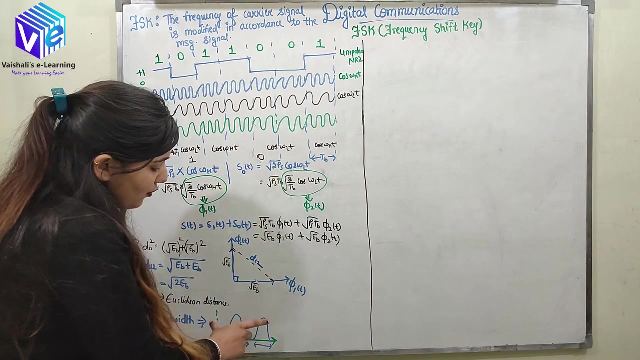 here I can see that Euclidean distance is under root 2EB. We use this Euclidean distance to find out the probability of error. So now coming to the bandwidth, So the output signal is comprised of two carriers, So it is having two carriers. 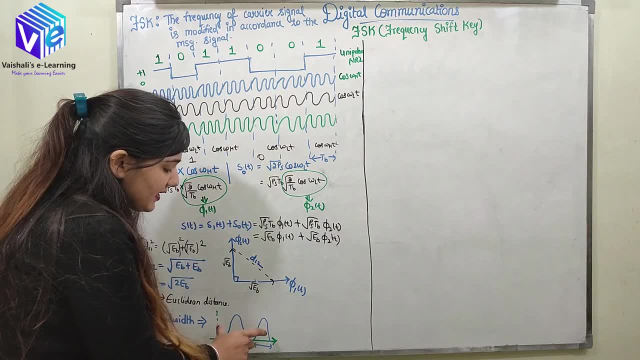 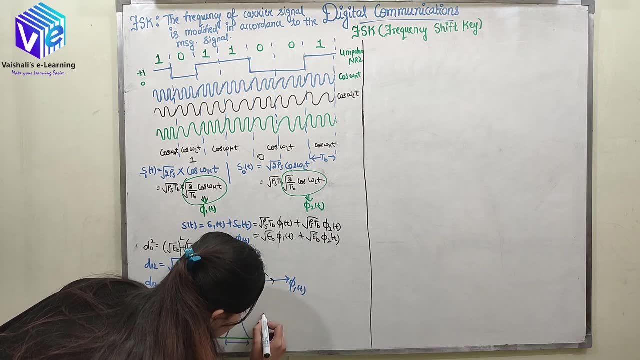 which are represented by the power spectral density, like this. So the two carriers are having the bit duration TB, So I can represent them with the Gaussian function and the bit duration for both of them is TB. So the distance between them, the highest and lowest part. 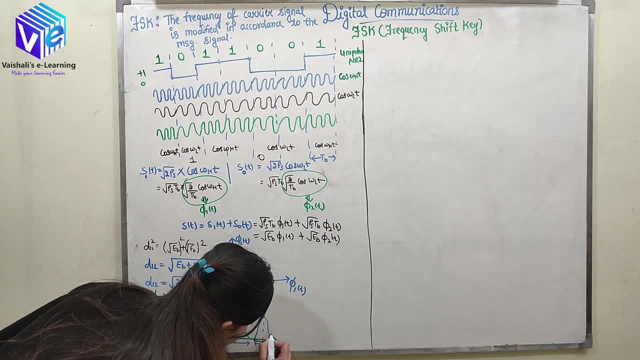 of the high carrier is 2TB, because this is FH plus FB and this is FH minus FB. Similarly, this is FL plus FB, this is FL minus FB. So this is FH plus FB and this is FL minus FB. So this is FL plus FB and this is FL minus FB. 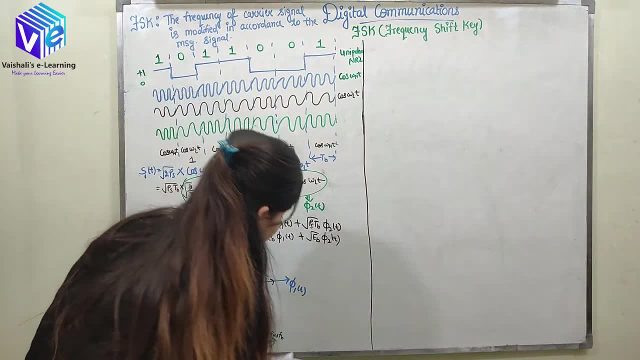 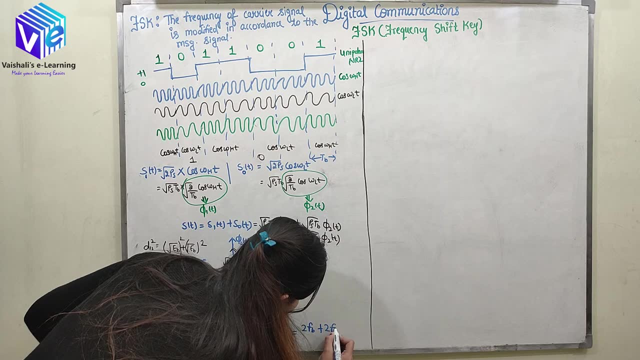 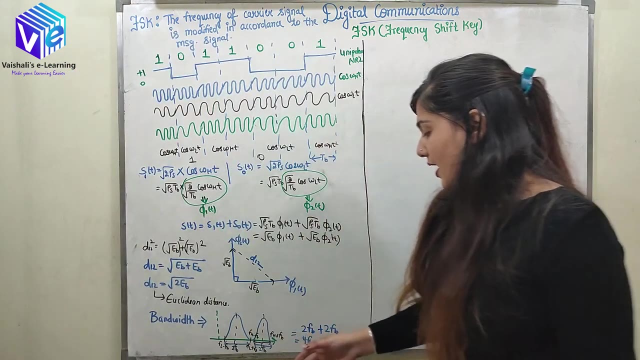 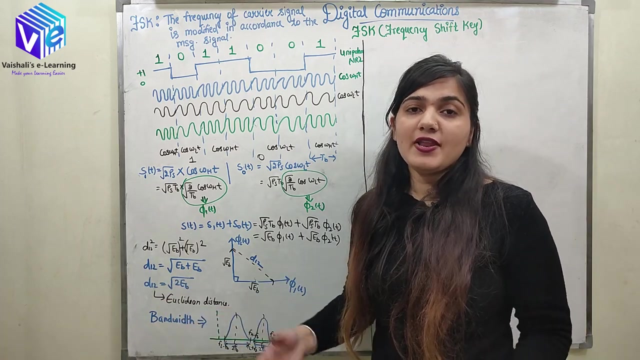 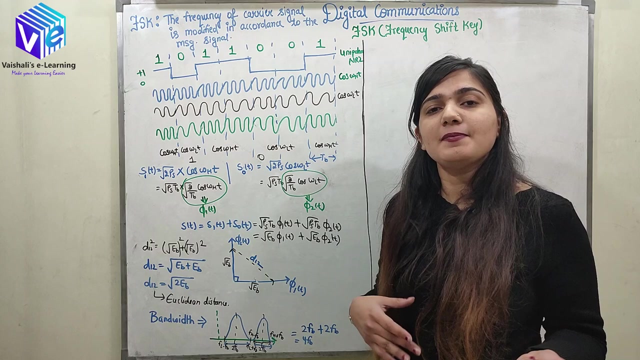 So again, this is so. the bandwidth is 2fb, So the bandwidth is 2fb plus 2fb, So bandwidth is 4fb. Now I can see the bandwidth has increased, but with the help of Euclidean distance. in the next video we will see and we will compare the probability of error of ASK, FSK and PSK. 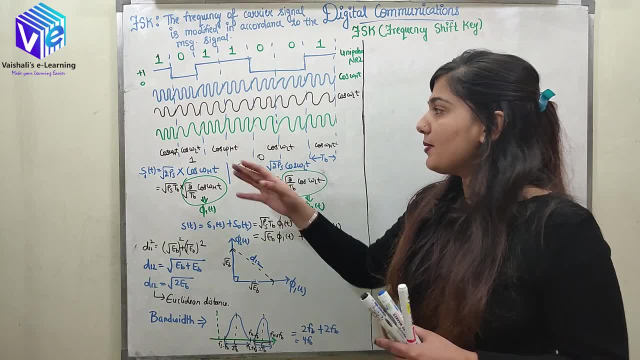 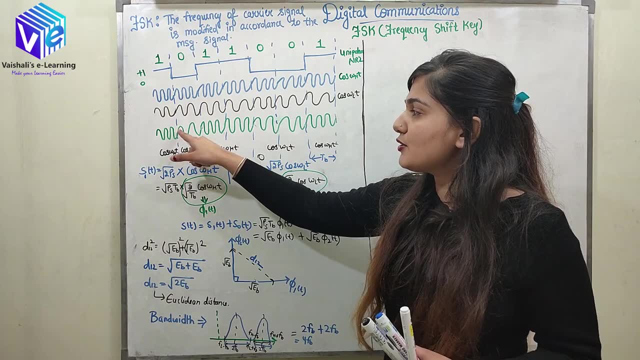 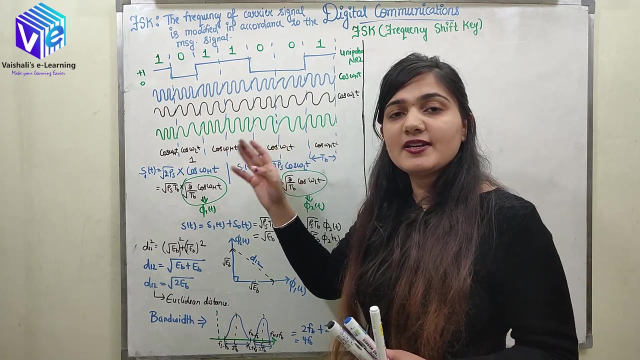 Then we will get to know why we are choosing FSK Plus. in FSK we don't have a DC component, so every time there is a signal. So in ASK, 0 was represented by 0 level. So if I have long stream of 0s, the long stream of 0s is represented by long 0s. 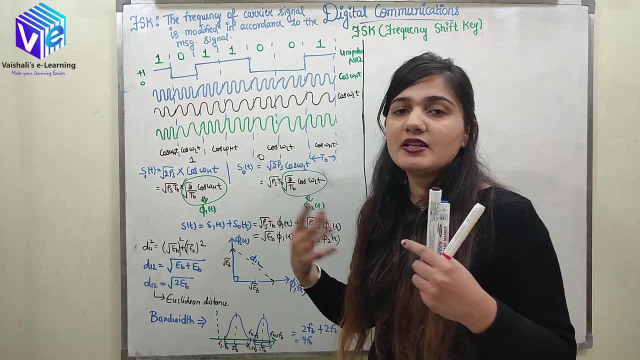 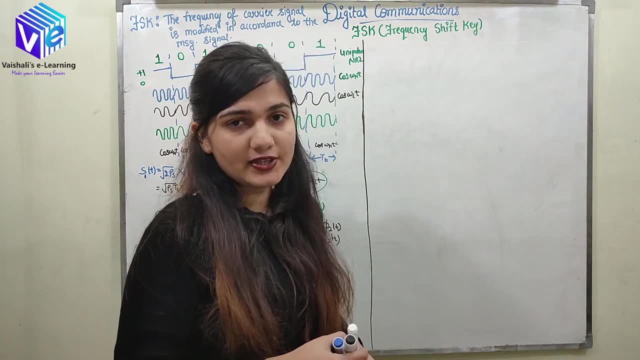 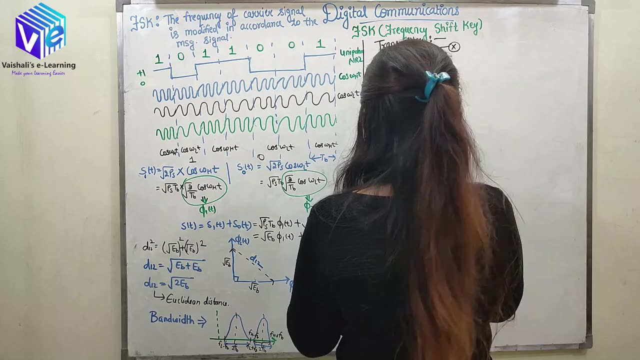 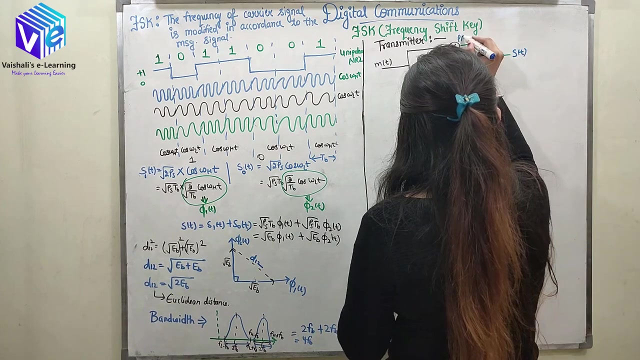 So the receiver would misinterpret that The signal is not coming. So to avoid all these things, I have FSK. So now coming to the block diagram of transmitter of FSK. So this is the block diagram of the transmitter. I hope now you understand what is happening. 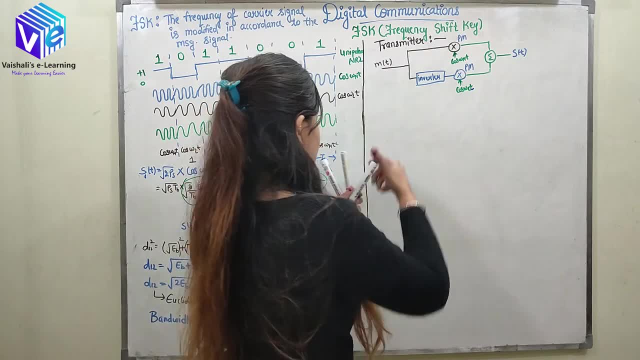 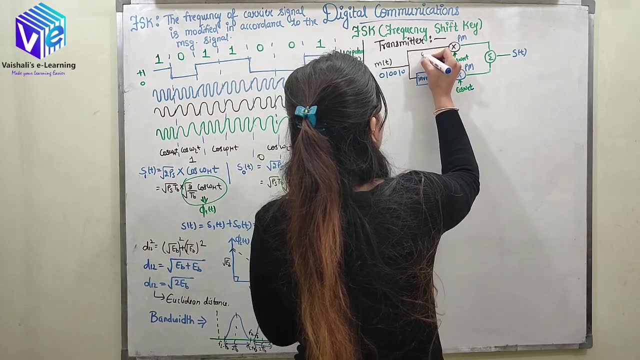 In the FSK. as you can see, the signal is not coming. Okay, so first I have the message signal, So message signal is represented like this. So if this is the message signal, so message signal is going here. So at the product modulator, the message signal is multiplied by cos, omega, ht. 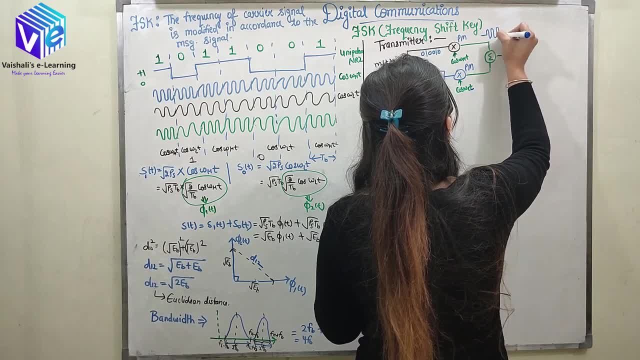 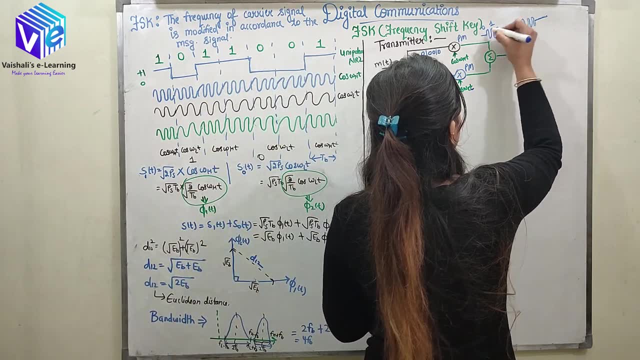 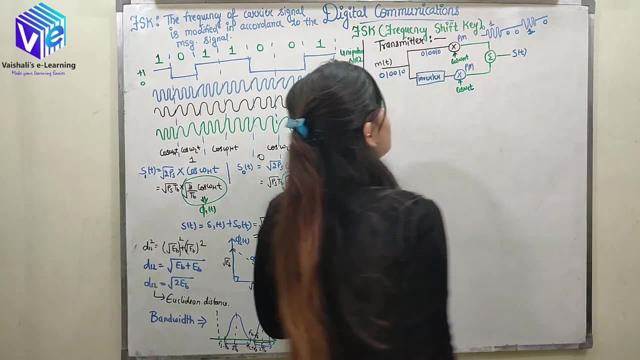 So here I will get a signal which is represented like this: at 0, 1, 0.. So 1 is represented by a high frequency carrier and 0 are represented by 0. So this is 1, this is 0. So this is how my output is represented at this block. 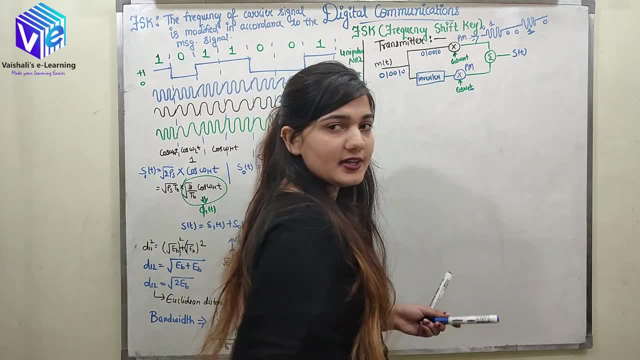 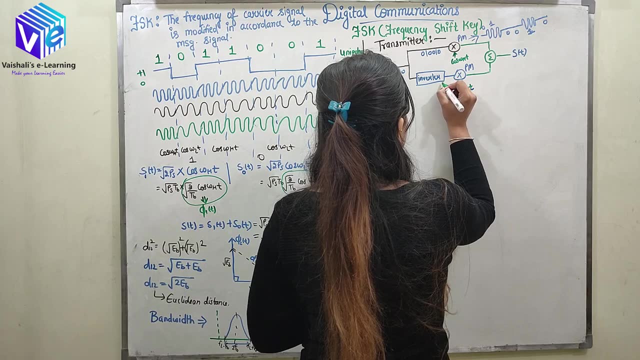 So now coming to the downside block. So here I have inverter. So at the inverter 1 is converted to 0 and 0 is converted to 1.. So now, after the output of inverter, I will get 0, 1, 0, 1, 1, 0, 1.. 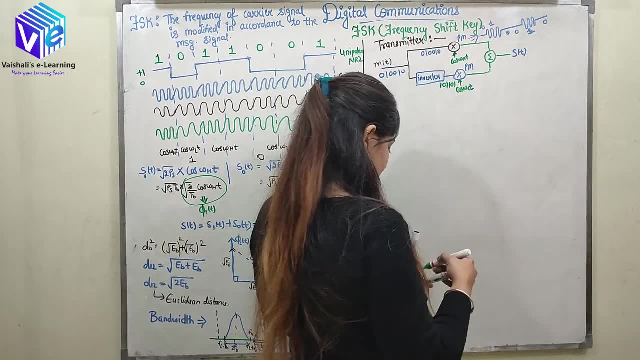 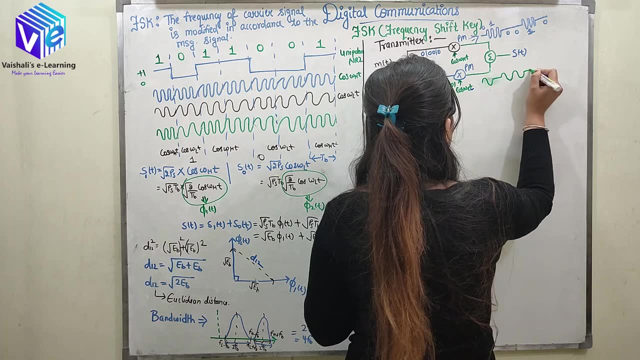 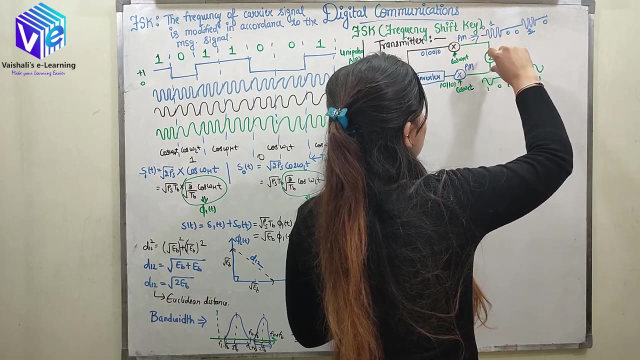 So the output is multiplied by low frequency carrier. So now I have 1. So this is 1.. So the output is represented like this: At first bit level I have here 0, I have here 1. So when these two are combined at first level, I will get this frequency. 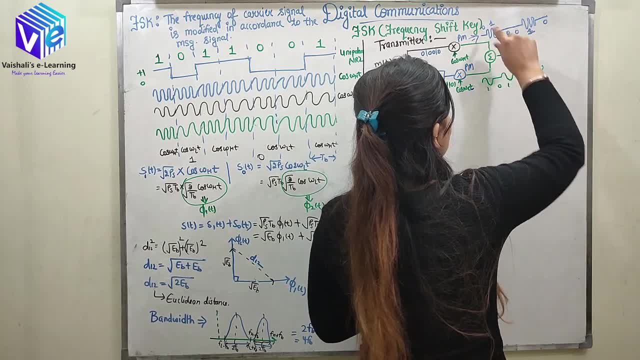 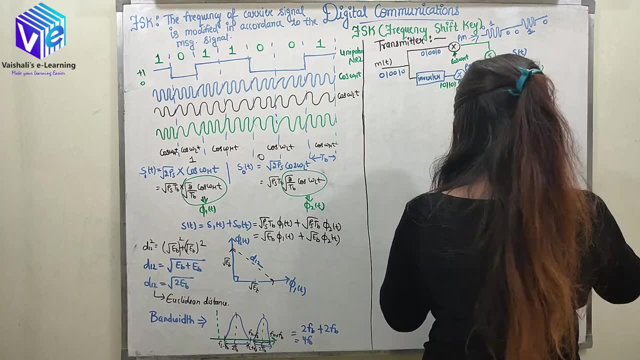 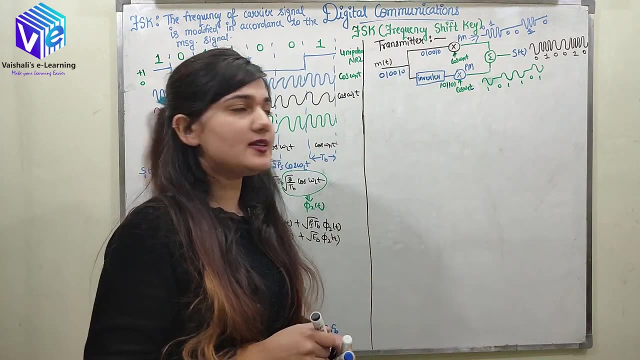 At second level. here I have frequency here 0.. So I will get this frequency. So when I combine these two, I will get the output which is represented like this: This is my output. So now you can see this block diagram is working in accordance to my FSK modulation scheme. 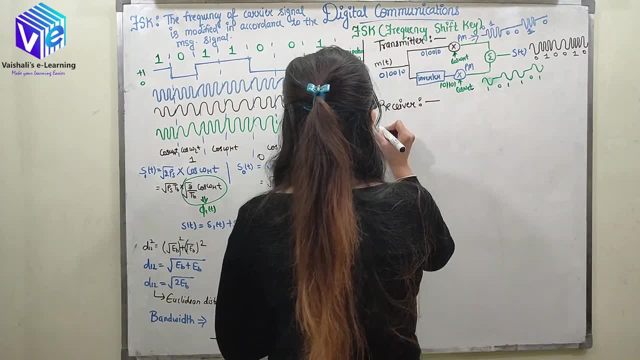 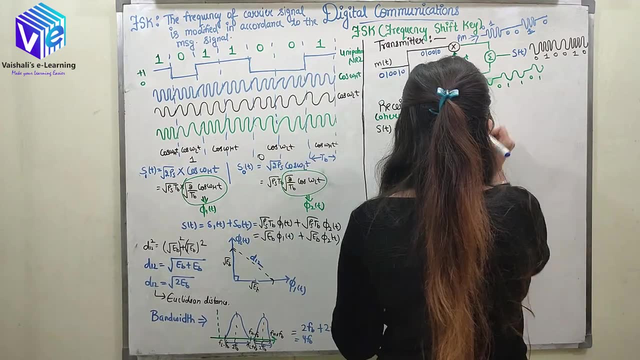 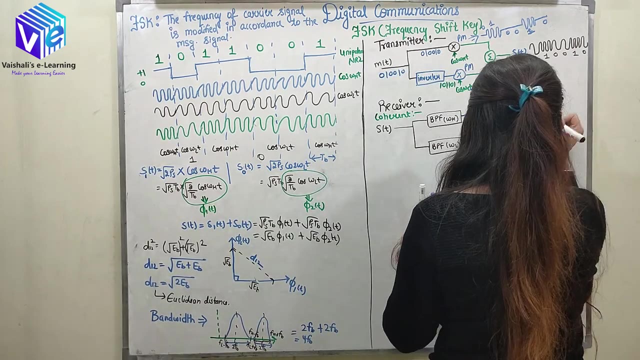 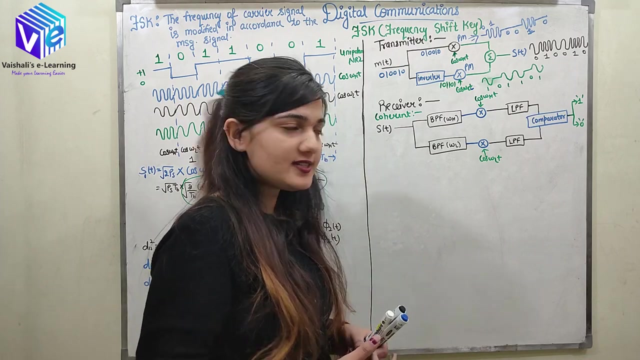 So now, coming to the receiver, Let's cross this out to our output. We will now be multiplying 1 by 1 to get what we want to get, And this is 1.. So 1, 1, 1, 0, 1, 2, 10 to 3.. 3 0 1 0 1 1 0, 1.. 2 0 1 0 1 0 1 1 1 2 1 2 1 11 0 1 0 1. 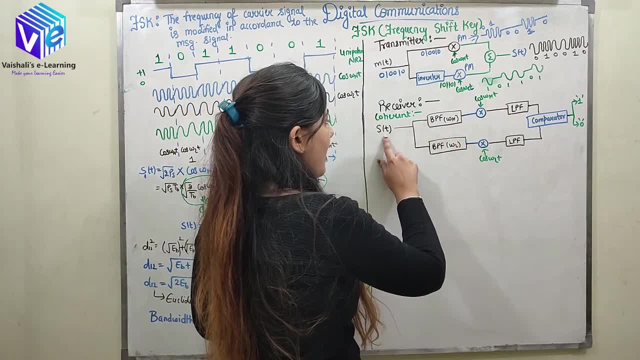 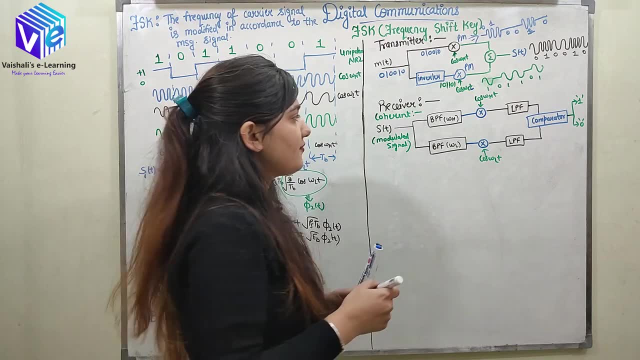 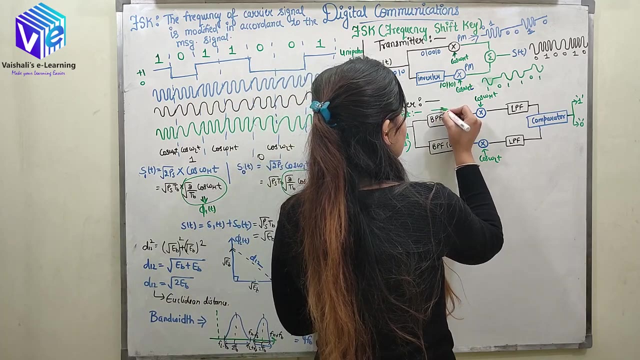 2, 1, 1 0, 1 0, 3 0, 1 0, 2 3 0, 1 1. So now I have the output modulated signal. So this is my modulated signal. So this signal is fed to the bandpass filter which is having the frequency omega h, So it is only transmitting the signal which is having the frequency omega h. 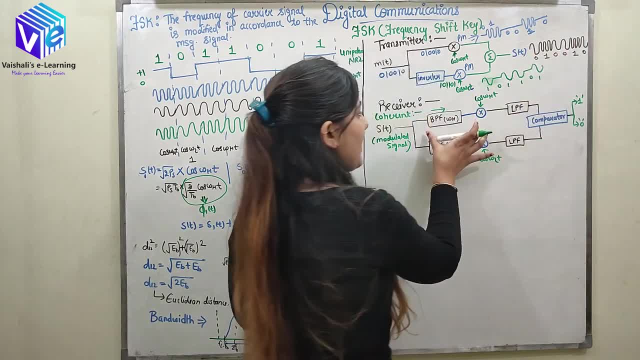 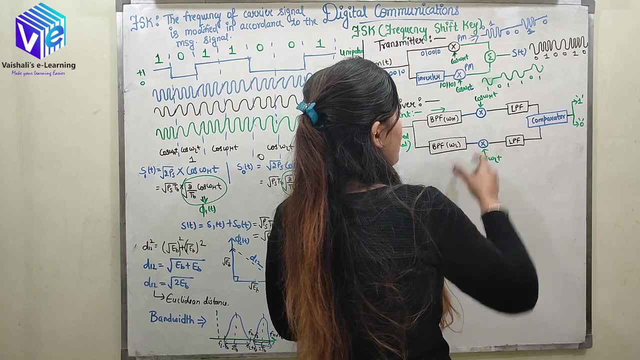 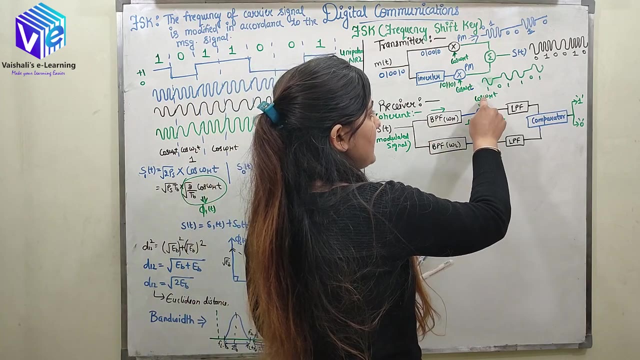 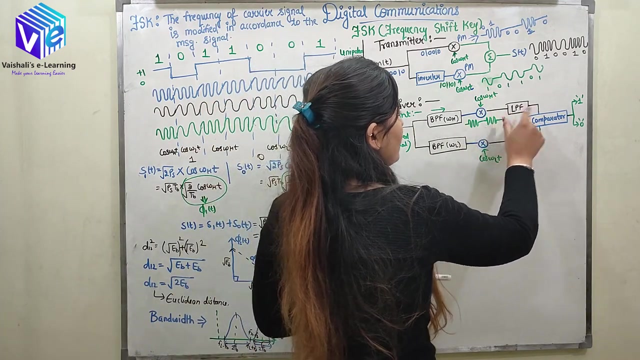 So now this is the signal. So with the help of bandpass filter I can eliminate all the low frequency components here. So the output of this bandpass filter would look like this: So now this bandpass filter is again multiplied by cos, omega, ht, So high frequency carrier is again multiplied with this. So after that, if I pass it through low pass filter- So I hope now you get it- 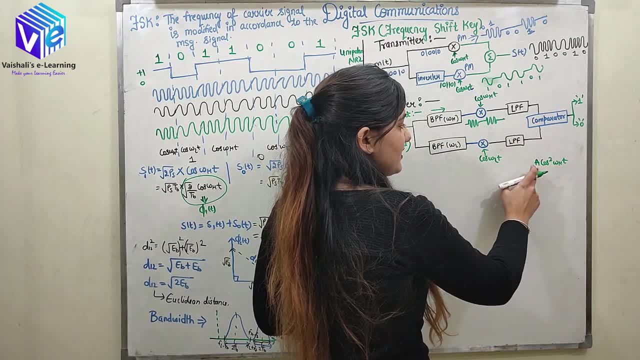 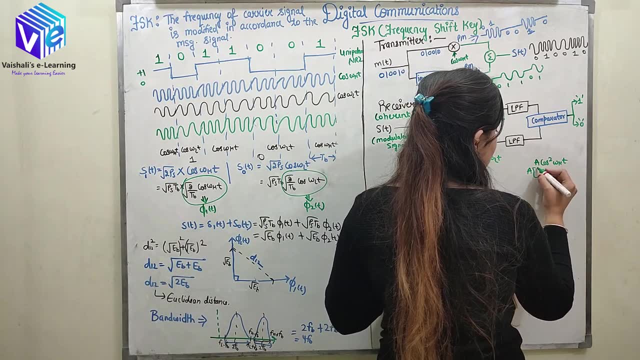 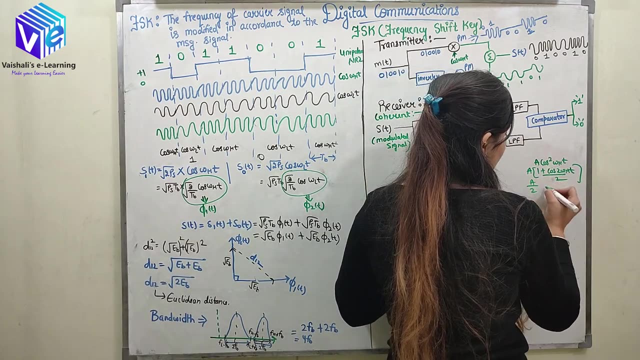 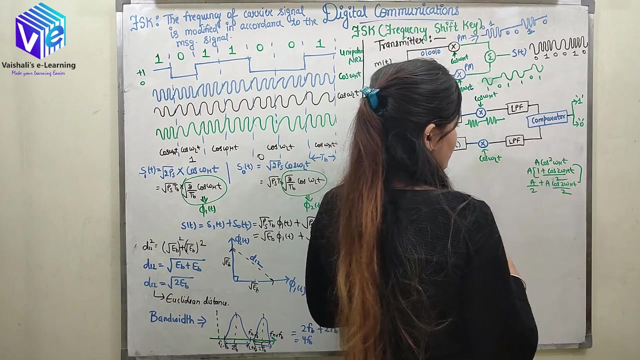 I will get A, which is the amplitude received, amplitude multiplied by cos square omega ht. So I can represent cos square omega ht as 1 plus cos 2 omega ht upon 2.. So after I expanded this, So now when I pass this signal through the low pass filter, this is my high frequency component. So this is get it rejected. 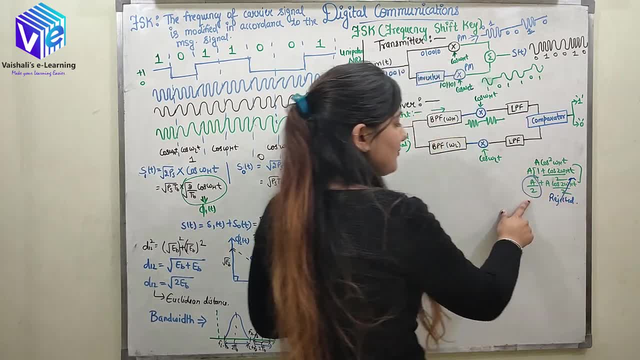 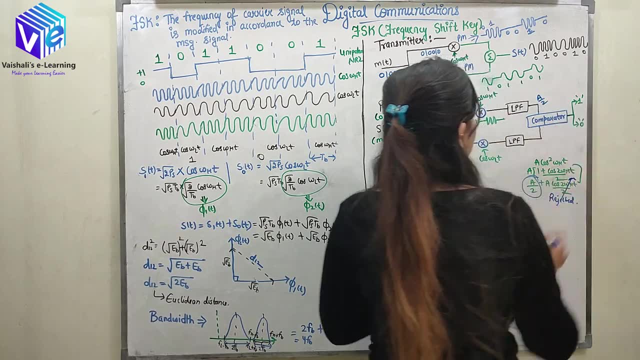 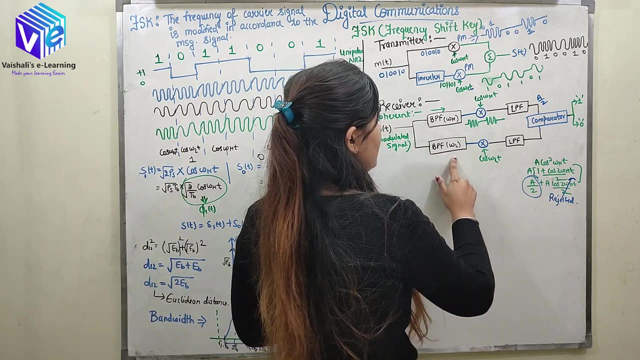 The high frequency signal is rejected and I am only left with the low frequency message signal. So at the output I am left out with A by 2.. So now again at the lower block I have the bandpass filter with omega ht. So here I will get all the low frequency components. 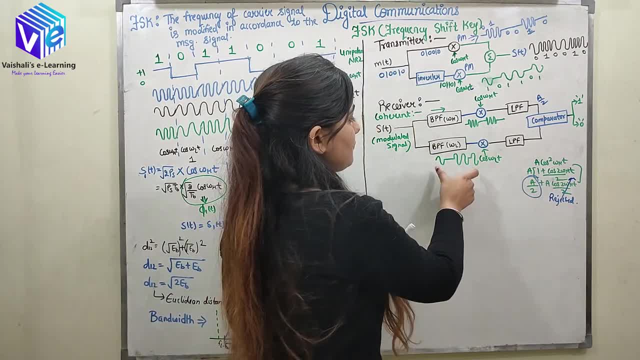 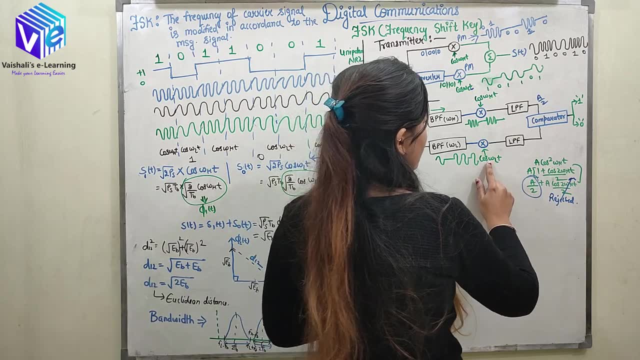 So this is how my output looks like. It rejects all the high frequency components from the output of ST. So this is how my output looks like. It rejects all the high frequency components from the output of ST. So, when it is multiplied by cos, omega, ht. So similarly, I will reject the high frequency components. 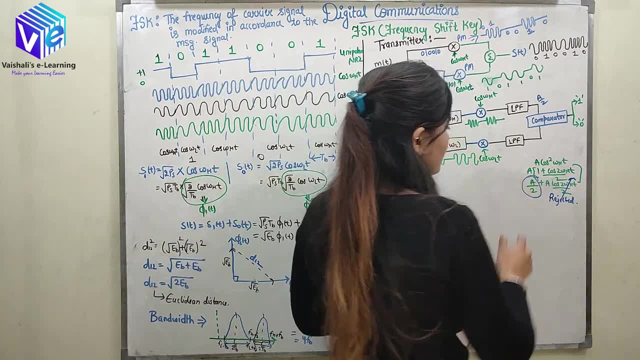 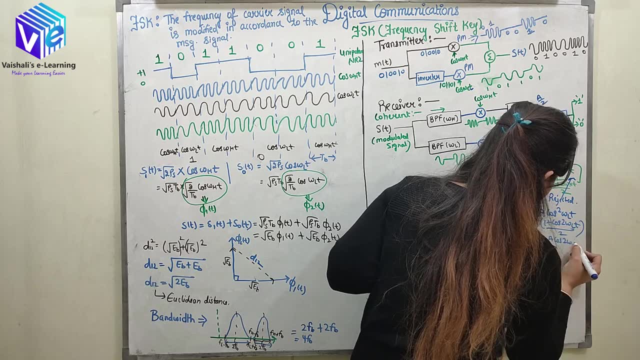 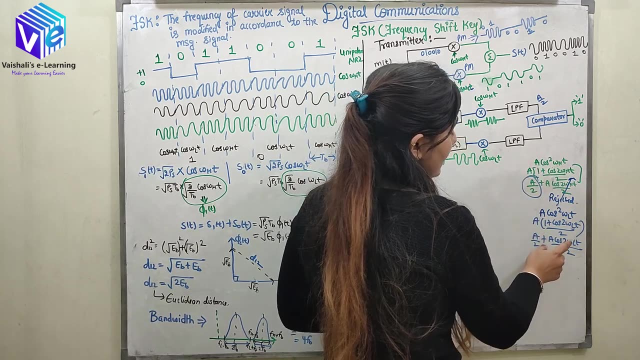 Remember, here I have cos omega ht, which is low frequency, So I will represent it as So. I have represented my signal like this. So after passing through low pass filter, this signal get rejected. Why I have written: it is A cos 2 omega ht. 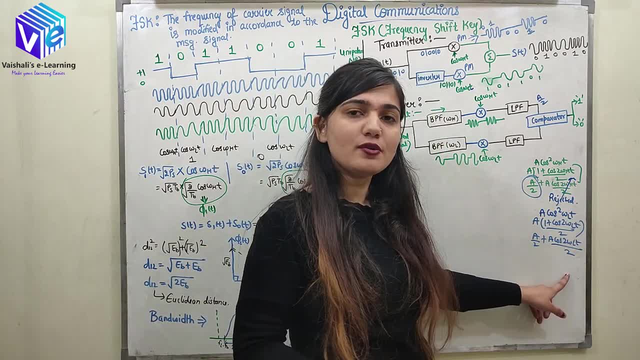 Why I have written it is A cos 2 omega ht. Why It rejects omega ht upon two. Why It rejects omega ht upon two. So it is also a low frequency component. So it is also a low frequency component, but it is a low frequency component of carrier. 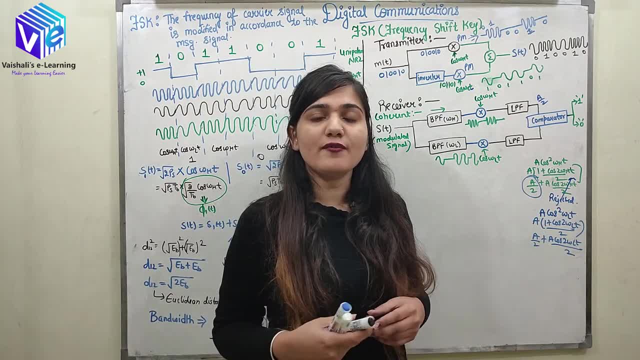 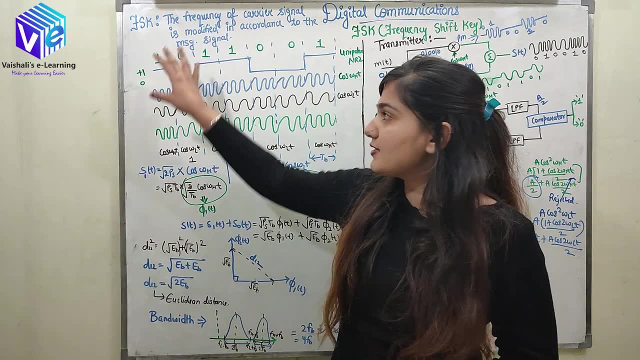 So we will understand this with the help of an example. So let's suppose you are walking and your speed is represented by the frequency of message signal. So your speed is the frequency of message signal. So I have two carriers now. 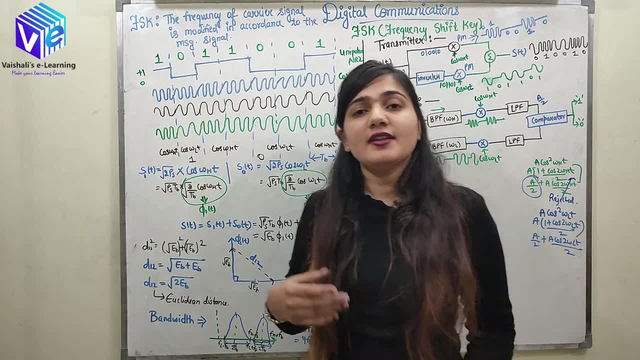 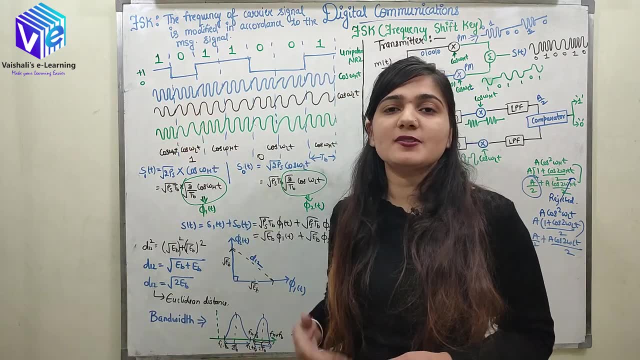 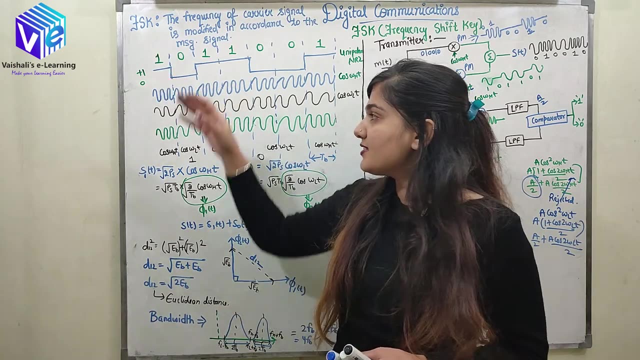 High frequency carrier and low frequency carrier. The high frequency carrier is the speed of an aeroplane airplane and the low frequency carrier is the speed of a train. So if you are superimposed on high frequency carrier, your speed would increase. Similarly, if you are superimposed. 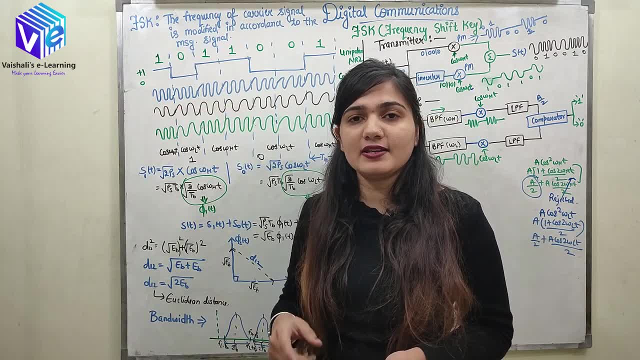 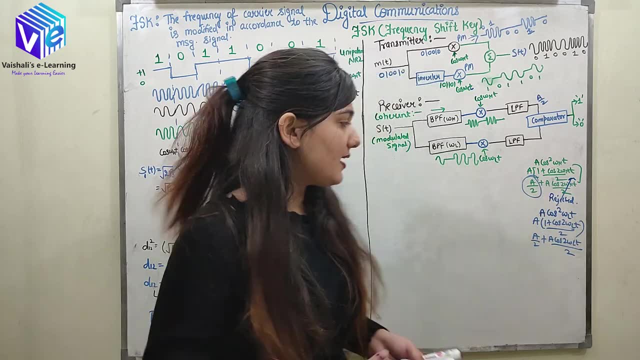 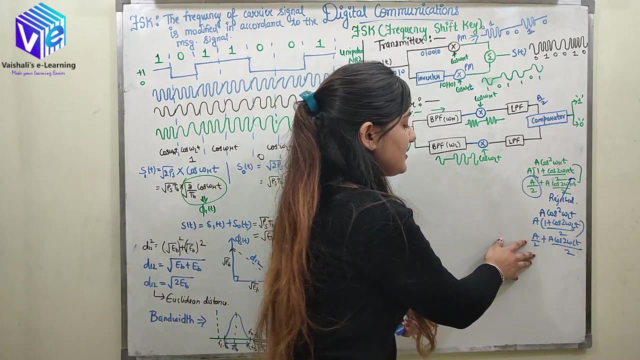 on low frequency carrier, that is, train, your speed would again increase. So the speed of train, when it is compared with your speed, it is very high. Similarly, the frequency of low frequency carrier is much high as compared to the frequency of the message signal. So 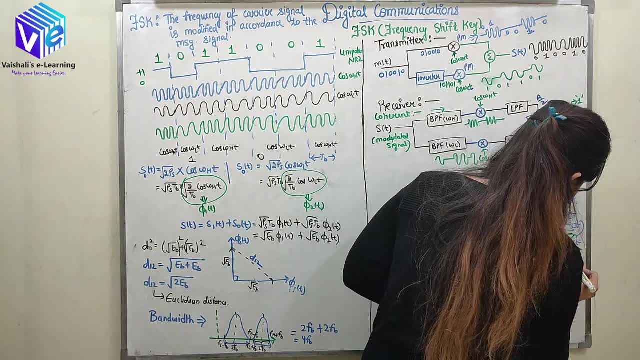 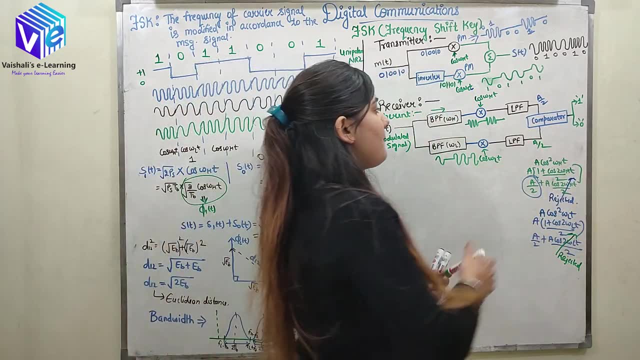 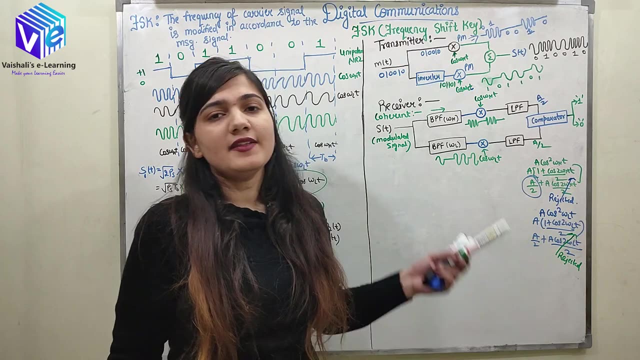 this is why this is also get it rejected. Similarly, at output of low pass filter, I am left out with A by 2.. Now the comparator or the decision making device will make the decision that I have 1 or 2 based upon the level of the amplitude of A by 2.. So I hope. 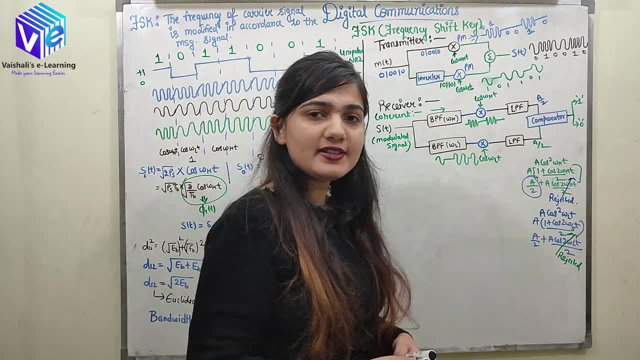 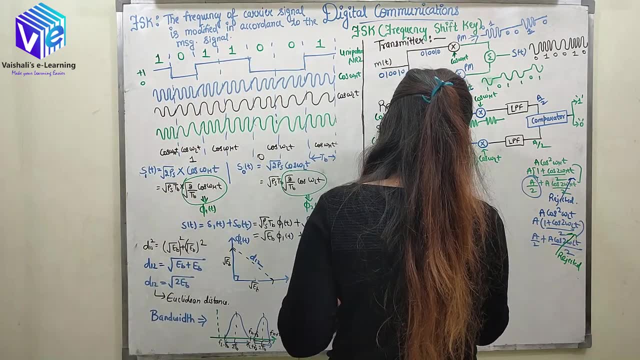 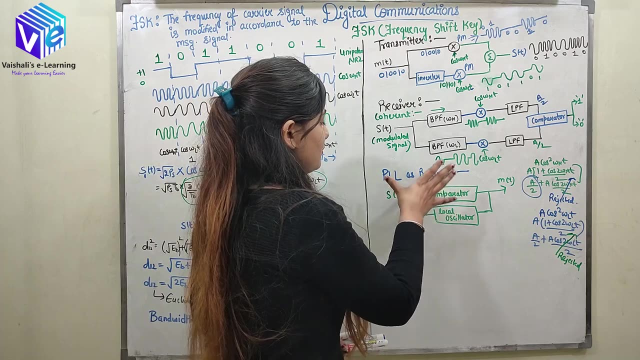 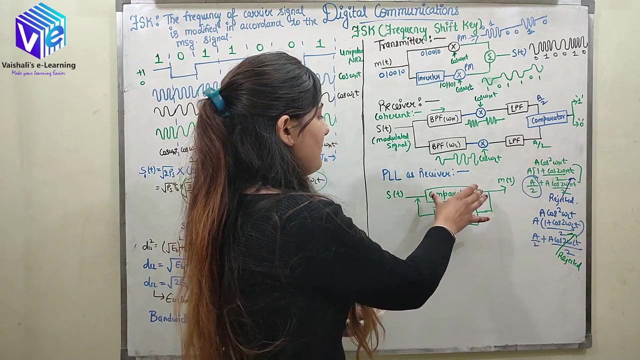 now you understood The basic functioning of the coherent receiver. Now we will come to the phase lock loop. So now, when I use the phase lock loop as a receiver- so it can be used in the case of FSK only- I have the comparator, I have the local oscillator in the feedback. So 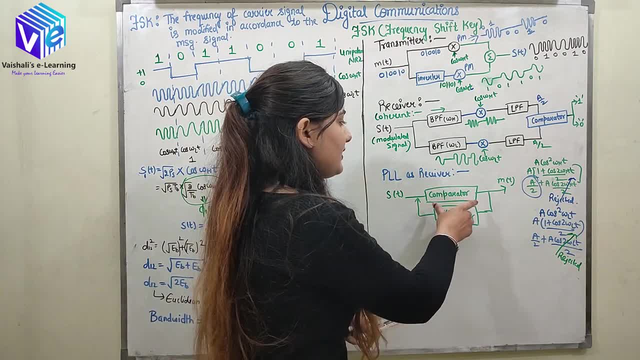 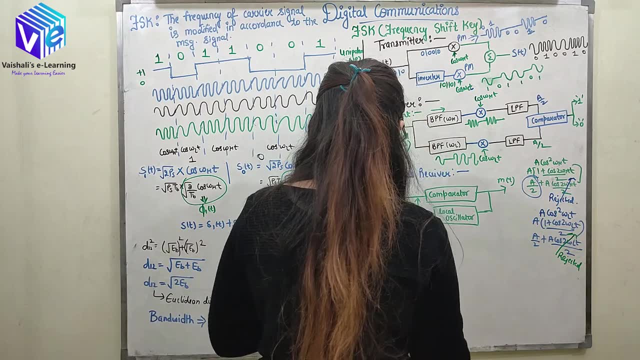 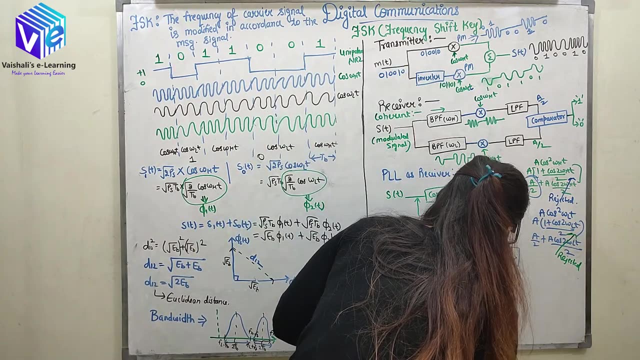 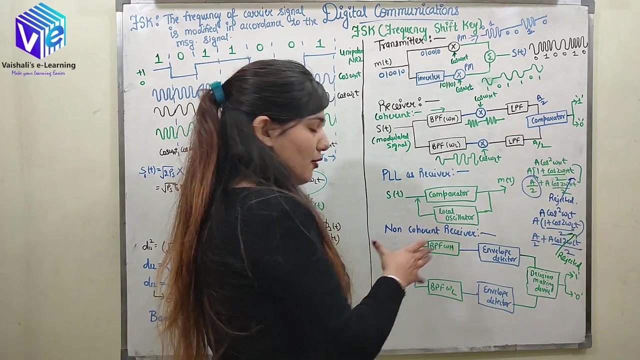 the local oscillator gives its value. I have the comparator which compares and gives me the message signal. So now coming to the non-coherent receiver. So now, in non-coherent receivers, I have the signal which is again passed to the bandpass.